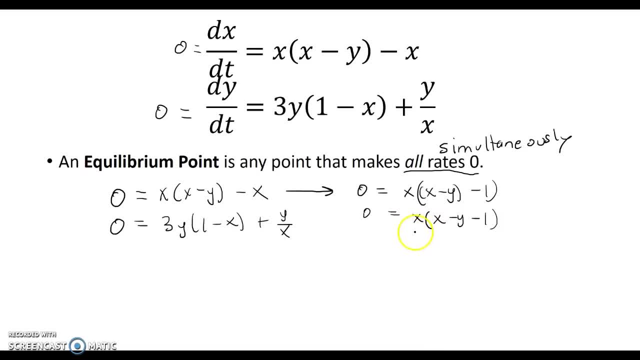 I have x times x minus y minus 1.. So this differential equation would be zero when either x equals zero. So when we're dealing with population, it's pretty common If you don't have a population size to begin with, you're not going to have any population change. 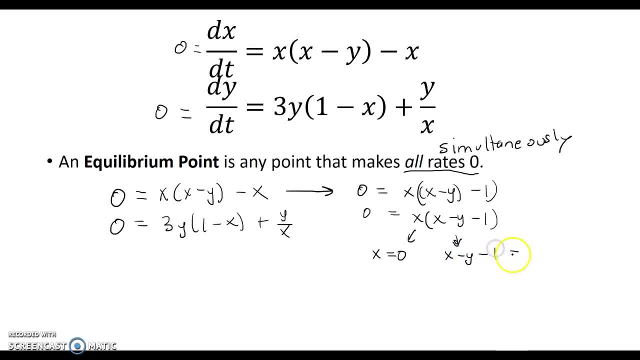 And similarly, here we have x minus y minus 1 equals zero. Now this is an equation that actually requires some work, So I can decide which variable I want to isolate here. Since I'm focusing on x, I'm going to isolate x. 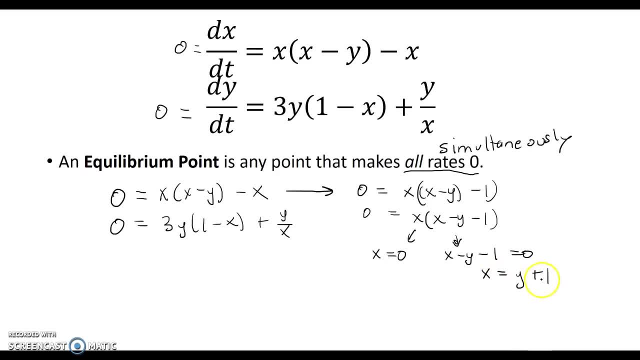 So if x is equal to y plus 1, or x minus y minus 1 is zero, this differential equation will also have a zero rate of change. Now it's not good enough. we said These are two possible equilibrium points. 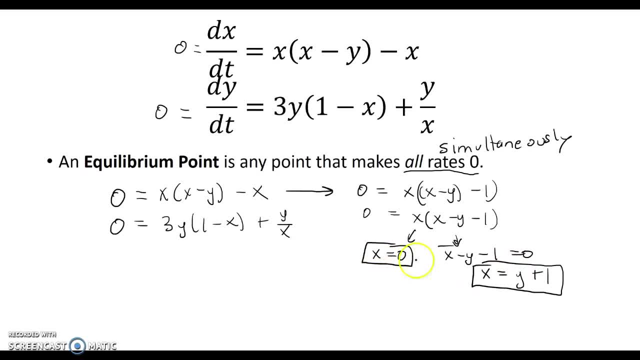 But these aren't really points. These are just single values of x that will make the first differential equation zero. So for the second equation, now we need to determine if x equals zero. what does y need to be in order for this to happen? 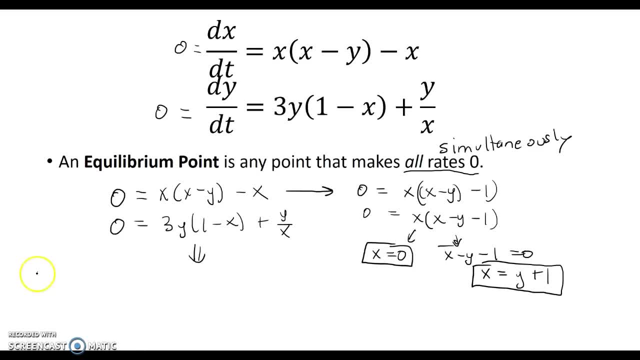 Well, so in this case we have, if we plug in for x equals zero. in other words, now we're going to figure out what corresponding y would be required in order to solve this equation. Well, we have, zero equals 3y. 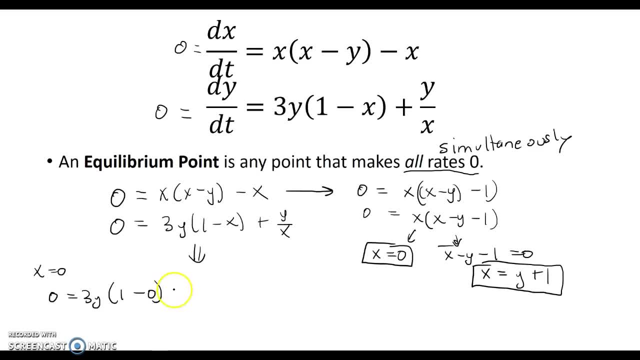 times one minus zero, since x is zero plus y over zero. But already we see a problem: We have a divide by zero error here, And so there is no value of y that will make this differential equation zero if x is zero. 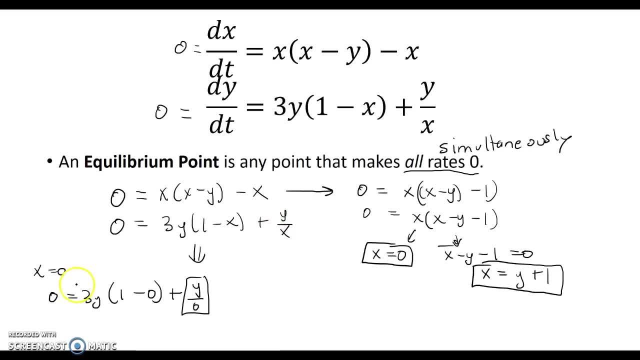 because x cannot be zero in this system. So we scratch that Now. if it were possible, if this were, for example, x over y, then this term would just be zero and we could proceed to solve for y as we tried. 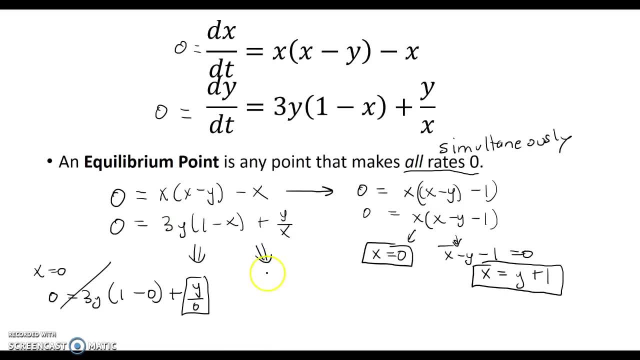 Okay, so now I need to also test this system. Okay, so I know that the first equation will be zero if x is equal to y plus one. So that means that zero is equal to 3y times one minus x. well, x is y plus one. 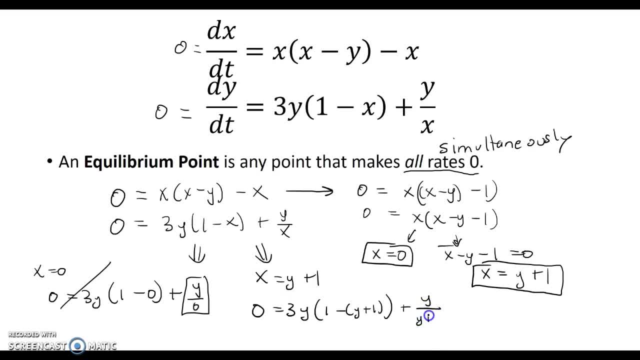 and plus y over x, which is again y plus one. So now I have to do some reduction and I see that I get 3y times one minus y minus one plus y over y plus one. Alright, well, this leads me to. 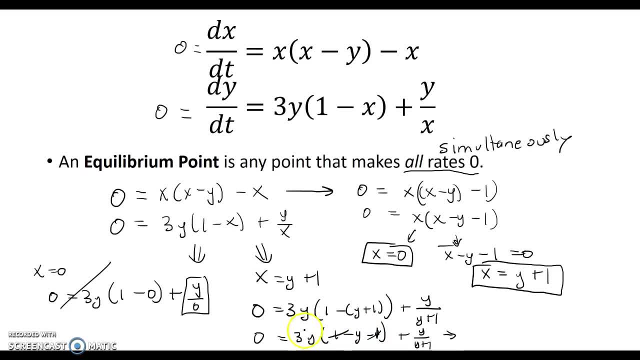 if I distribute well, actually I can cancel out a one and a negative one here, and then I'll have 3y times y, which is so I have. zero equals 3y squared plus y over y plus one. Okay, well. 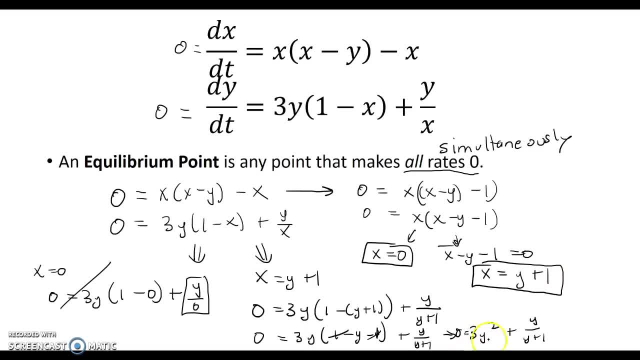 it might be obvious at this point that one of the solutions or one of the values of y that will work here is: y equals zero, because if y is zero, this first term will be zero and the second term will be zero. Moreover, what I can even do here is: 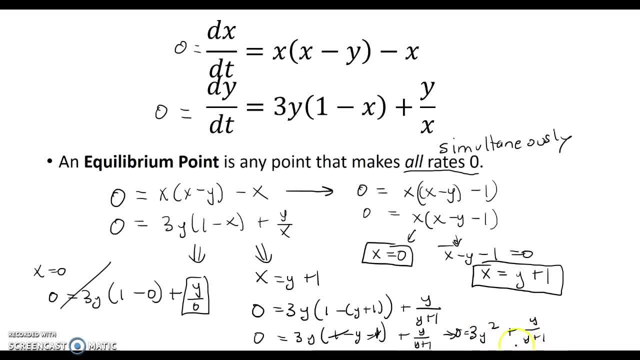 okay, so I need to solve this. I see that it's a quadratic. Now I know that y plus one cannot be zero, so y cannot be negative one here, And I need to keep that in mind if I'm going to do something like. 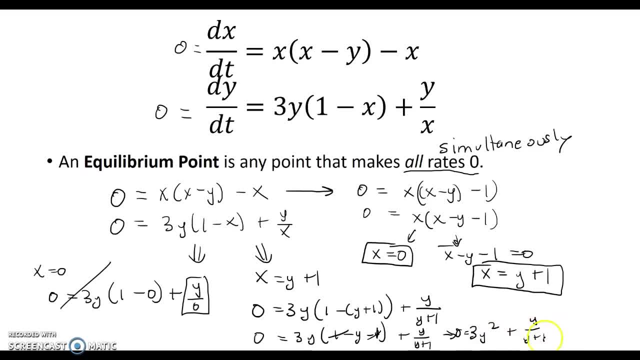 multiply both sides through by y plus one. But actually what I'm going to decide to do here- and I'll start back up here- is I am going to factor out a y from both terms and I'll have 3y plus one over y plus one. 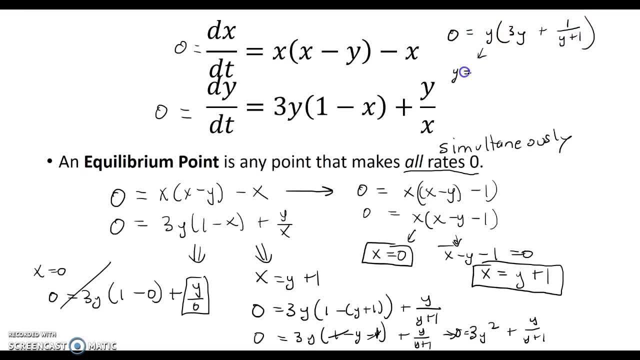 Okay, well, there it is. There's the y equals zero value. that will work and that doesn't cause any problems anywhere throughout the equation. because I won't be dividing by zero, I'll have zero plus one in the denominator, which is fine. 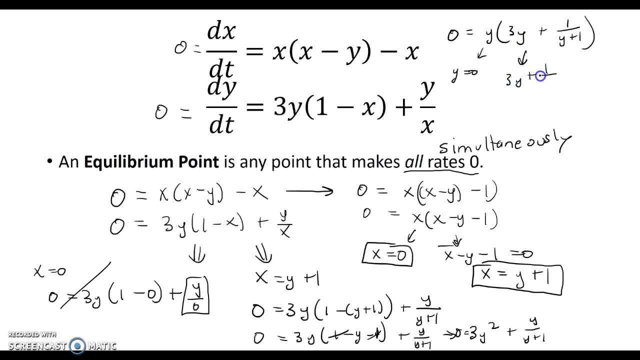 Or it could be the case that 3y plus one over y plus one over y plus one equals zero. So let's just point out here: we observed that y cannot be negative one, and so if we do accidentally get y equals negative one. 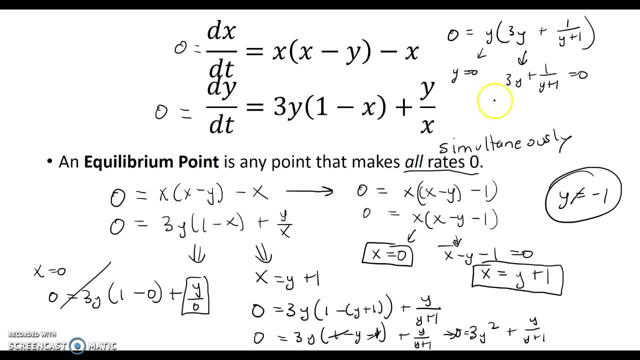 we'll have to deal with that. Okay, so now I'm actually going to go ahead and multiply through by y plus one, multiply both sides by it, So I'll have y plus one times 3y. and if I multiply one over y plus one by y plus one, 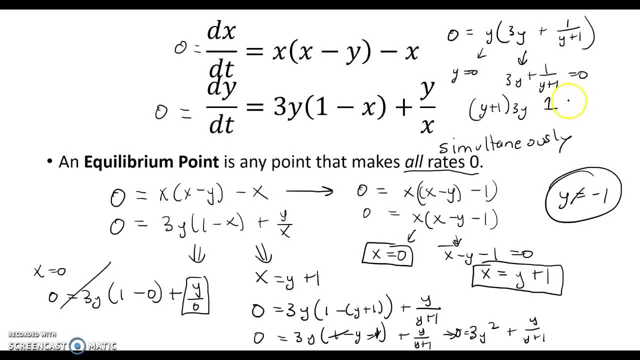 I'll just have one, because the y plus ones will cancel and I'll have that equals zero. Alright, I'm going to move over to this side. I didn't realize I would require this much space, And now I have. well, I can't really do much here. 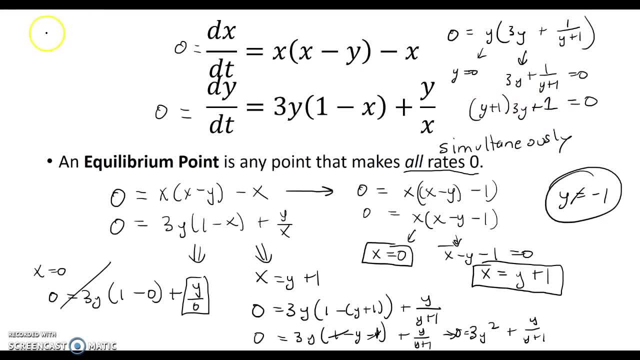 because this is not all multiplied together. so I am going to redistribute again and I'll have 3y squared plus 3y plus one equals zero, And then you can see that this is quite non-trivial. In other words, now we have to solve a quadratic. 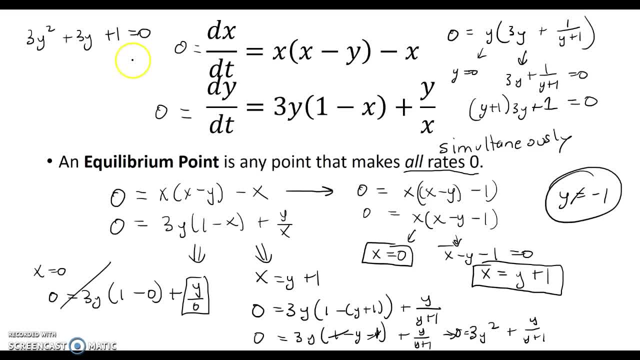 to figure out any values of y that will make that second component zero. So there's one solution. So if x is equal to y plus one, y has to be zero, and if y is zero, that means x has to be one. 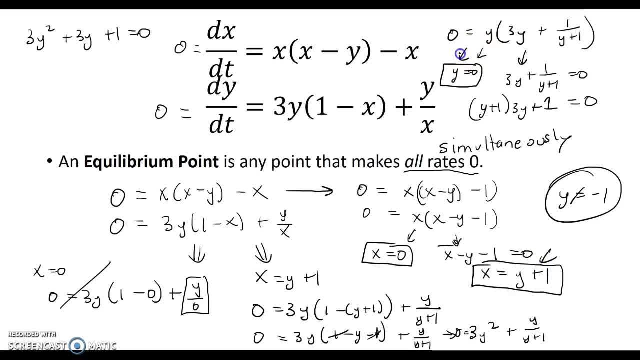 So it's kind of like we have to keep in mind that this is the guy that gave us this guy. And to solve this, what I'm going to do is I'm going to divide both sides by three, so I have y squared, plus y plus one third equals zero. 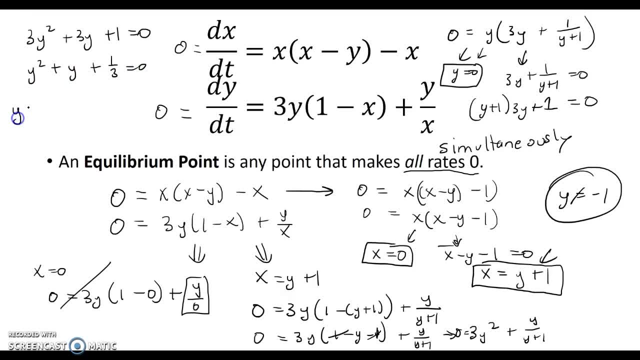 And now, using quadratic formula or using a calculator, I would have the value of y that's satisfied is negative b, which is one plus or minus the square root of b squared, which is one minus 4ac, which is four times one times one third. 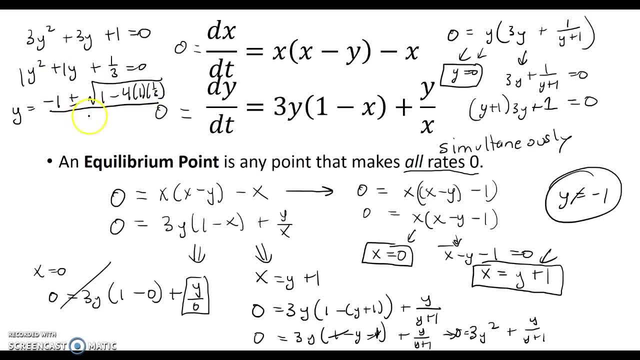 And that's all over 2a, and now a is one, so I have two times one, And so if I continue reducing this, I'll have negative one plus or minus Now under the radical. if I get a negative, I know that there will be no real y that will work. 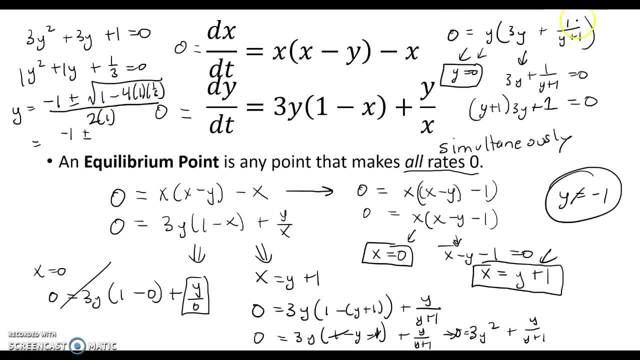 So that will work. That will tell me that the second term can never be zero, And let's see what happens. So we get one minus four thirds, which is one minus. well, one is three thirds, four thirds. that's going to leave me with a negative one third. 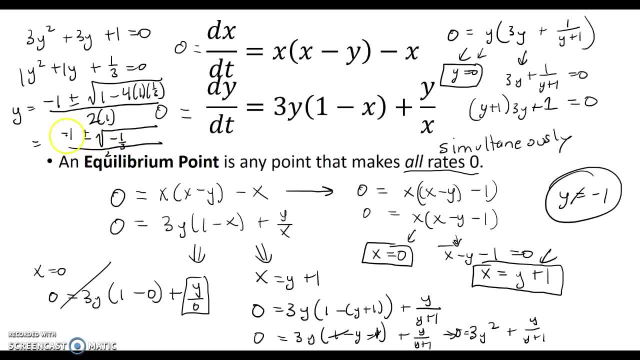 in the denominator all over two, and there is no real solution. y is not real. Okay, What did we figure out? Well, when x is zero, there is no corresponding solution to the second equation. In other words, although x equals zero. 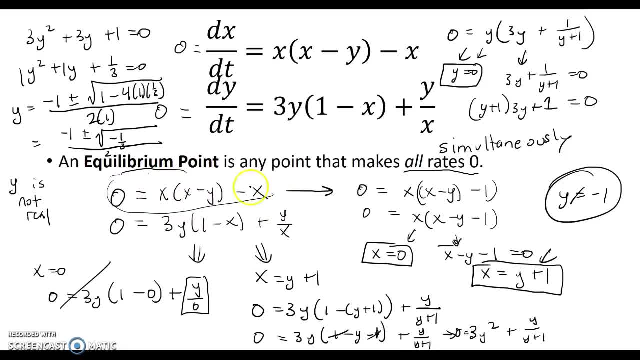 makes the first rate of change equal to zero. it does not in any way, possibly mathematically, allow us to make the second equation zero, because simply x cannot be zero. Then we decided: okay, well, the other possibility for the first equation. 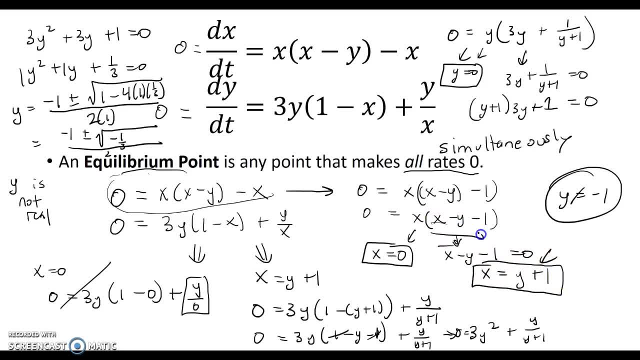 is, if x equals y plus one, then that means this component here in the parentheses will cancel to zero and will leave us with a zero in there. Okay, well, if that value of x works for the first equation, let's go to the second equation here. 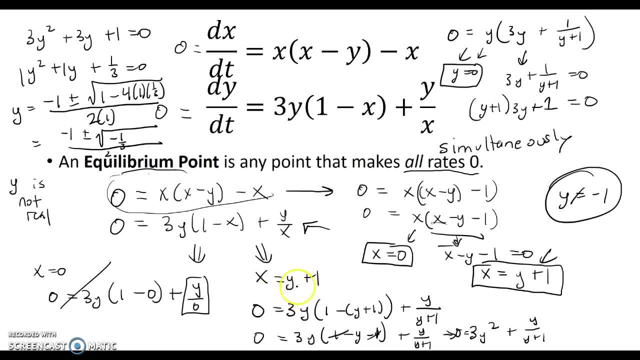 and solve that, given that x is equal to y plus one. And we did all this algebra here and found out that that's the same thing as solving: zero equals three y squared plus y over y plus one. And then we did some factoring. 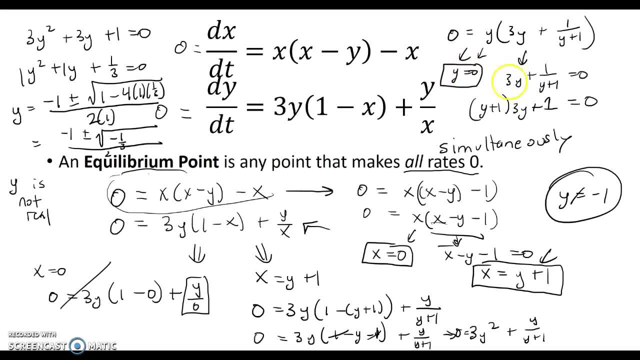 so that we could immediately obtain a solution: y equals zero, or three y plus one over y plus one equals zero. And so then we solved this component, which led us to a quadratic, and the quadratic led to negative, under the radical which said: hey, you know what? 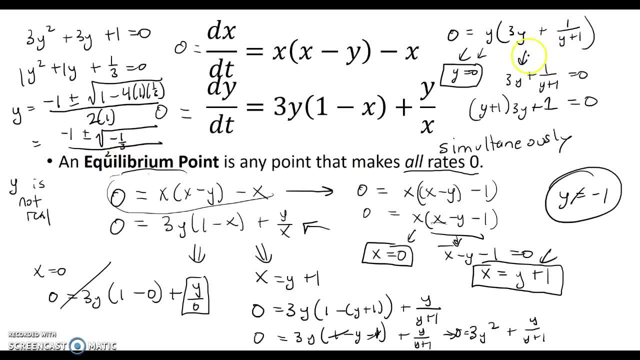 the second factor cannot be zero if x is equal to y plus one. So what solution do we end up with? Well, we ended up with this one here, right there, and that corresponded to this solution. So that was our only equilibrium point. 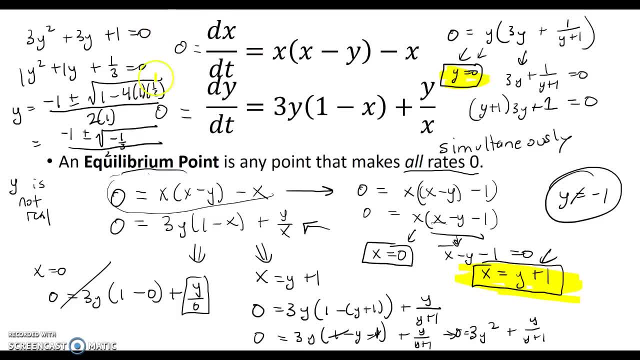 Now you can see how we could have ended up with more, quite possibly, if there had not been these issues of having y over x. similarly, if the square root here were not negative. Okay, so I'm going to move to the next page. 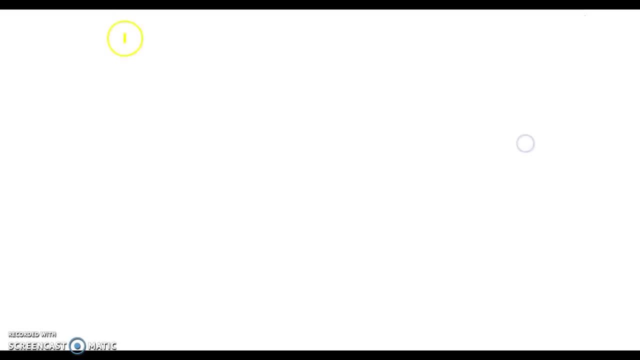 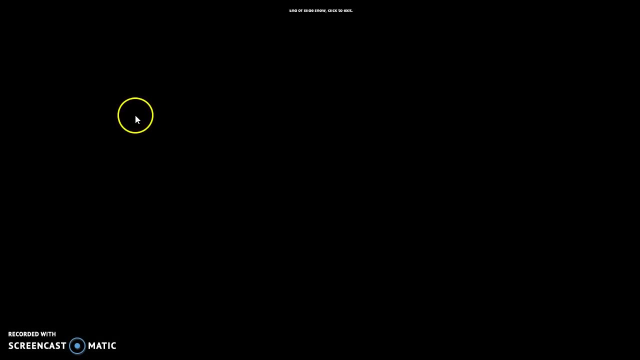 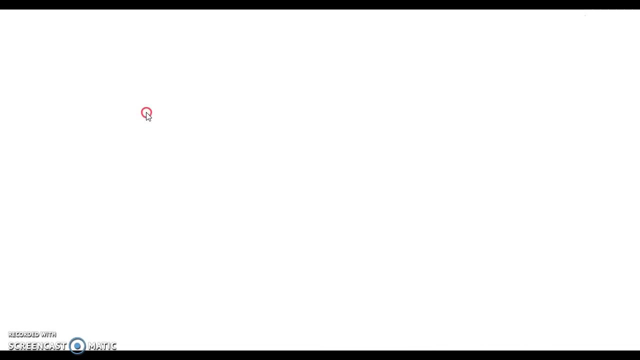 and we now know that y is equal to zero. Excuse me, I need to change my pen here. So we know that if x is equal to whoa- Sorry about that, folks. So we know that if oh boy. 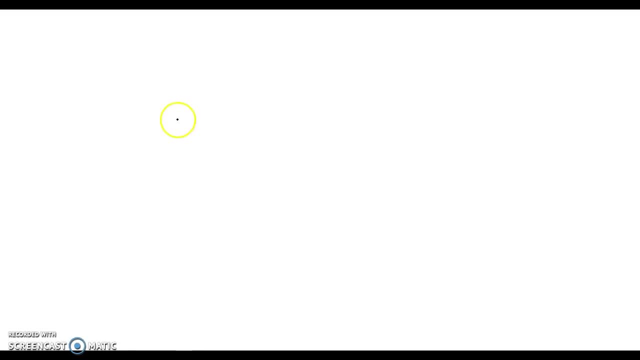 this is more trouble than I thought it would be Okay. so the solution that we found is: x equals y plus one led to the second equation, giving us the corresponding y value of y is equal to zero. Okay, well, that's the only equilibrium point.